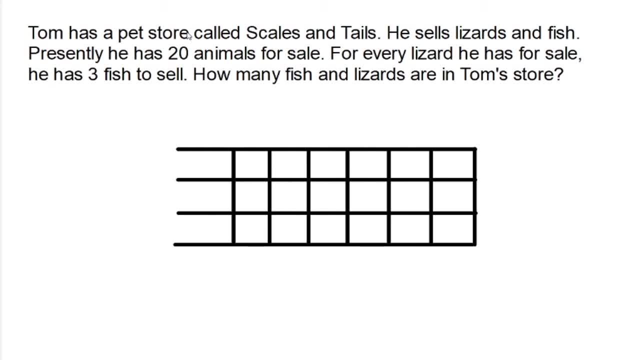 table. we're going to need three rows. we're going to need one row to keep track of how many lizards he has. we're going to keep another row to keep track of how many fish he has, and in our third row we'll keep track of the total pets. it says he has three fish for every lizard, so let's figure. 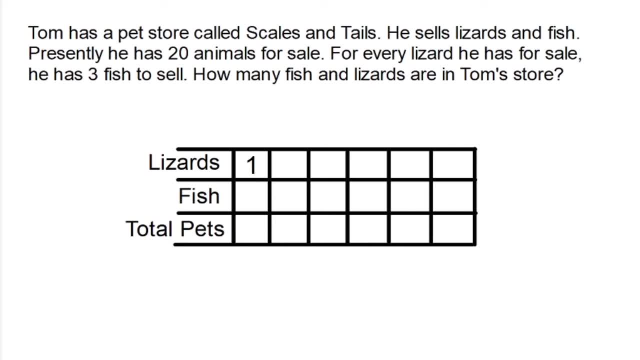 this out. if we got an animal for sale, we could keep track of all the homeless. do you know that? do if he has one lizard? what does that mean? How many fish? It says for every lizard, he has three fish. What would that mean? in total pets, Four total pets. So now we're going to continue. 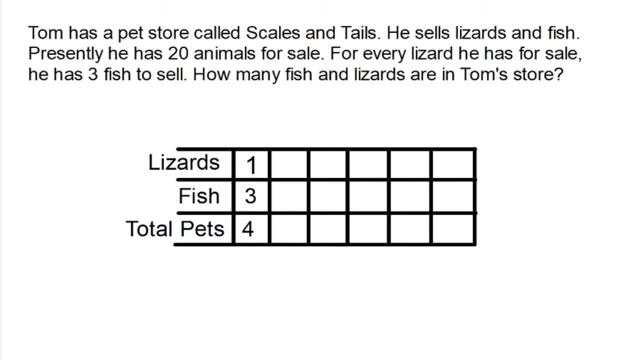 to fill in our table until we have enough information to solve the problem. So let's go. If he has two lizards, that means he must have six fish, And in that case two plus six would be eight pets. Okay, eight is not enough. He has 20.. So let's go on Three If he has three lizards. 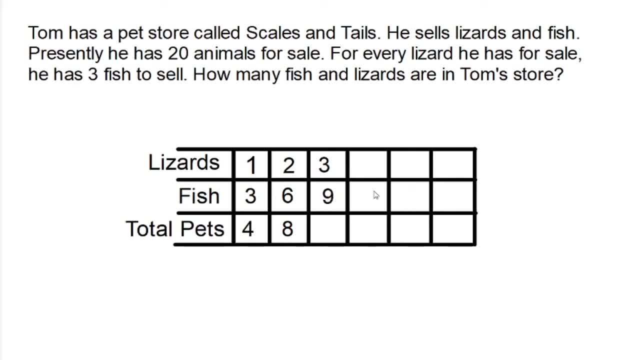 that means he's going to have nine fish, And that would mean he would have 12 pets for sale. Again, we have not yet solved our problem, So let's continue With four lizards for sale. he would then have 12 fish for sale And that would give us a total of 16 pets. 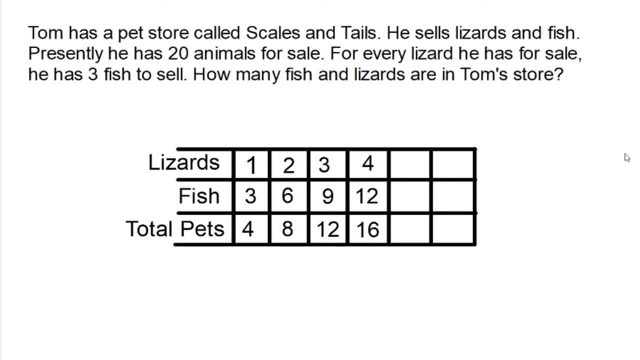 Still not enough, So we continue. If he has five lizards, that would mean he would have 15 fish And that would give us a total of 16 pets. So let's continue. And that would mean he would also have 20 total animals for sale. Well, it says in our problem. 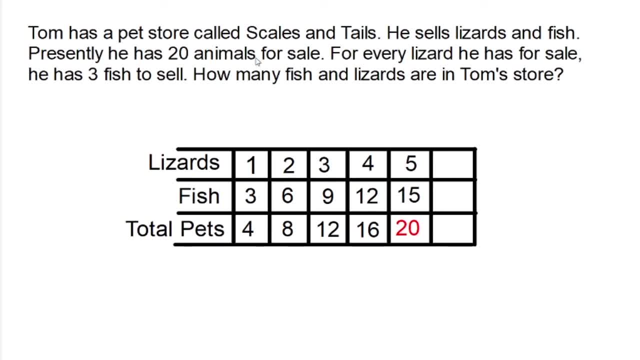 that he has 20 animals for sale. So our table is complete. We have enough information to solve the problem. So what is it asking us? It's asking us how many fish and lizards are in Tom's store. So, with the table filled, we can now solve our problem. Tom has five lizards. 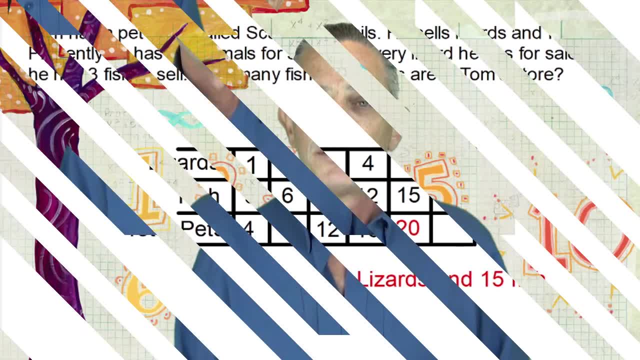 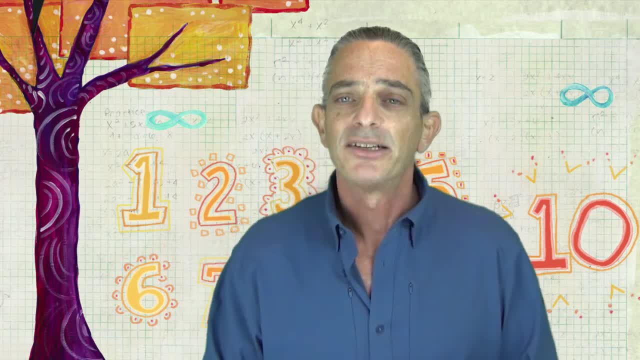 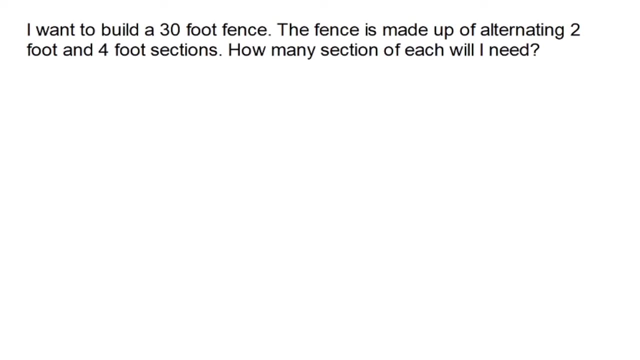 and 15 fish for sale. You see the way we organize that data into a table and then use that table to solve the problem Here. let's take a look at yet another example. Here we go. Let's look at this problem. It says I want to build a 30-foot fence. 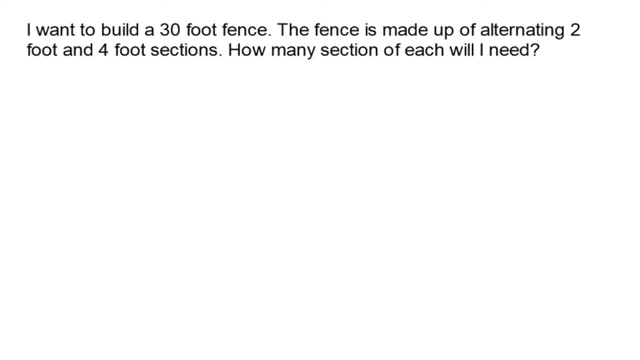 The fence is made up of alternating two-foot and four-foot sections. How many sections of each will I need? And the problem is telling us that I'm building a fence. I need to build 30-foot of fence. The fence is going to be made up of a two-foot section. 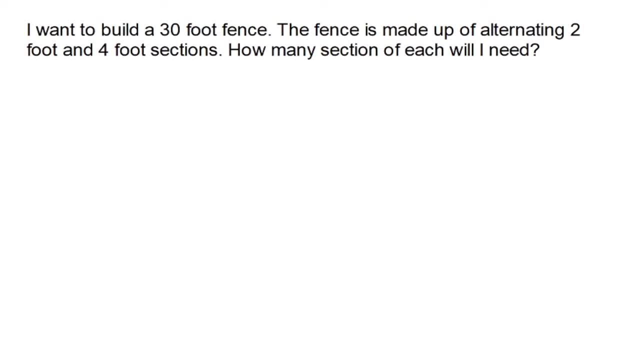 followed by a four-foot section, followed by a two-foot section, followed by a four-foot section, and it's going to repeat this pattern until I have all 30 feet. So let's solve this problem using the make a table problem solving strategy. So the first thing I'm going to do is make a table. 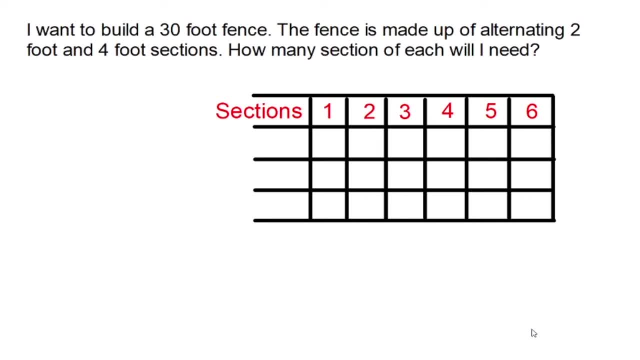 This table has four rows. The first row will keep track of the sections that I'm going to need. The second row is going to keep track of how many feet the two-foot sections take up. The third row is going to keep track of how many feet the four-foot sections take up. 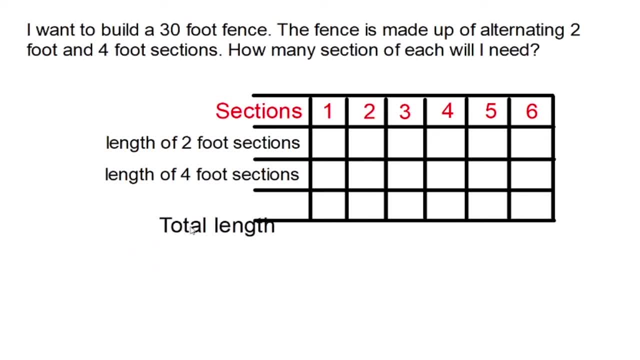 And the fourth row is going to keep track of the total length of my fence. And this fourth row is very important because when the total length is 30, I know I'm done Alright. so if I use one of each section, that means my two-foot sections are going to take up. 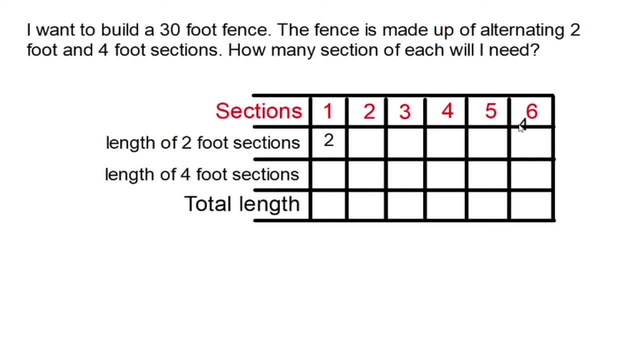 a total of two feet and my four-foot sections will take up a total of four feet. That's one of each. My fence at this point will be six feet long. Now if I use another section of each, you'll see I get an exponential increase of my other parts. 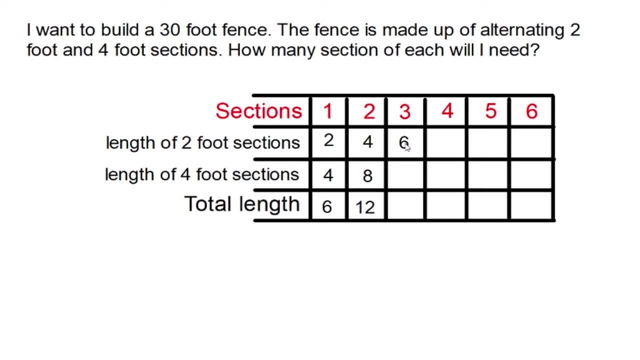 up to a total of seven feet. So, and if I use each section of each, I'm going to go back up a total of 40-feet. At this point you'll see, as a total total length of the fence will be 12 feet. 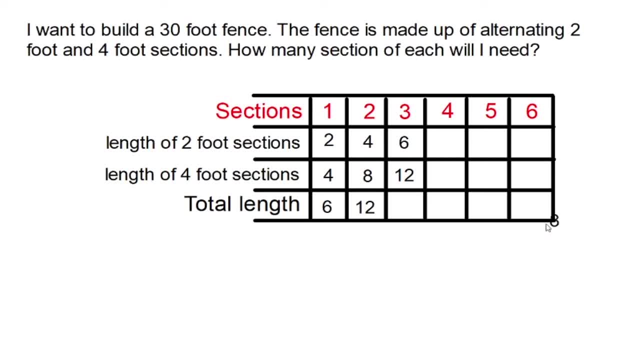 We'll take up 50-feet. If I use three sections of each, my two-foot sections will take up six feet. My four-foot sections will take That would be a total length of 18 feet. If I use 4 sections, my 2 foot sections will take up 8 feet. 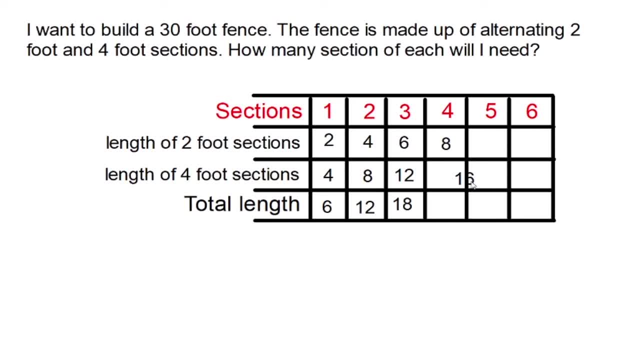 My 4 foot sections will take up 16 feet, and that would be a total of 24 feet of fence. If I use 5 sections, my 2 foot sections will take up 10 feet, My 4 foot sections will take up 20 feet and that will be a total of 30 feet altogether. 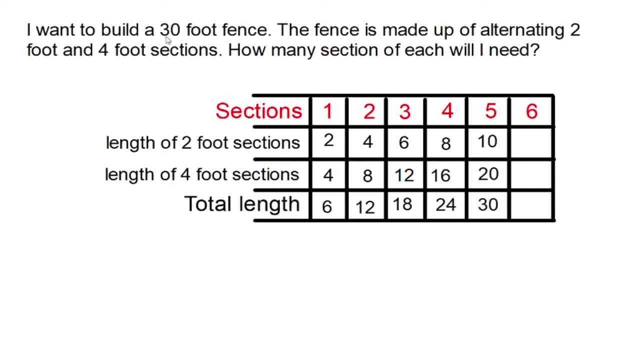 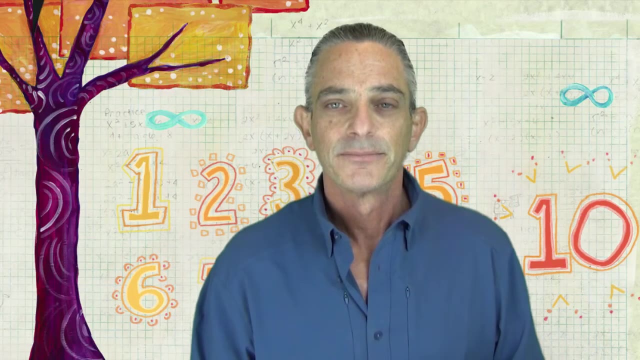 Now, 30 feet is exactly what I'm looking for, because I'm building a 30 foot fence. So I have now solved my problem. To make a 30 foot fence, I will need 5 sections of each: 5 2 foot sections and 5 4 foot sections. 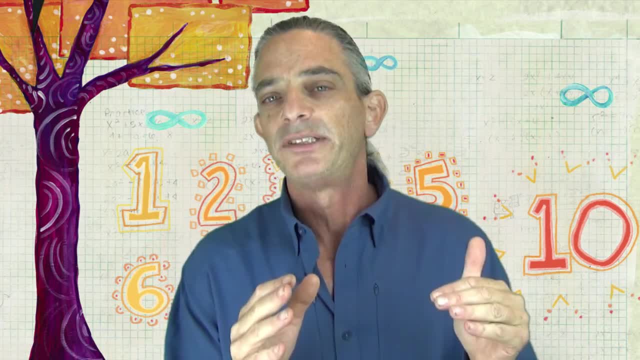 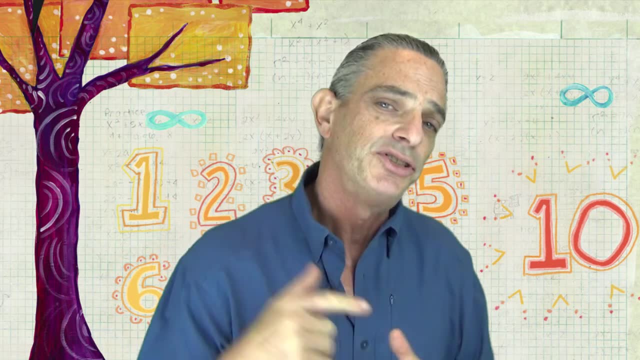 So once again you saw how we organize the data in the form of a table and then we use that table to solve the problem. So here let me give you an example and see if you can use the make a table strategy to solve a problem on your own. 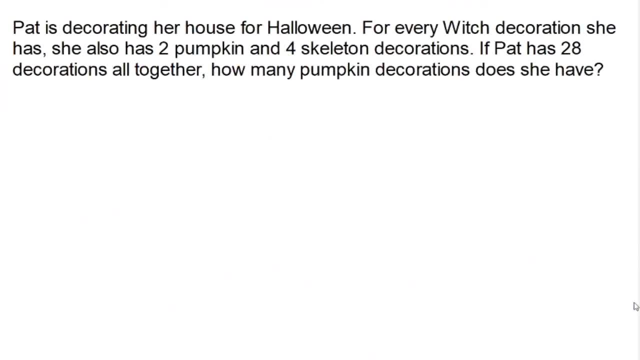 Okay, So here's a problem for you to try on your own. It says Pat is decorating her house for Halloween. For every witch decoration she has, she also has 2 pumpkin and 4 skeleton decorations. If Pat has 28 decorations altogether, how many pumpkin decorations does she have? 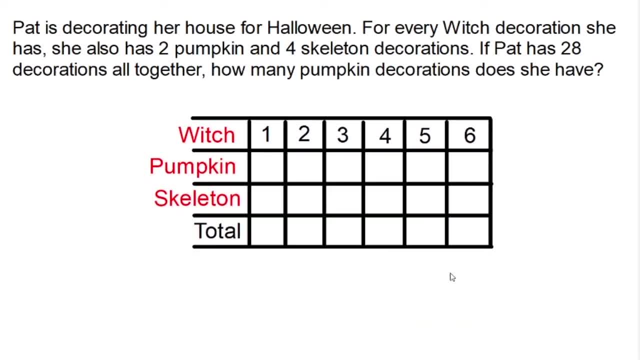 So to get you started on this problem, I went and built the table for you. In this table we have 4 rows. It's going to keep track of the number of witch decorations, the number of pumpkin decorations and the number of skeleton decorations, as well as the total decorations. 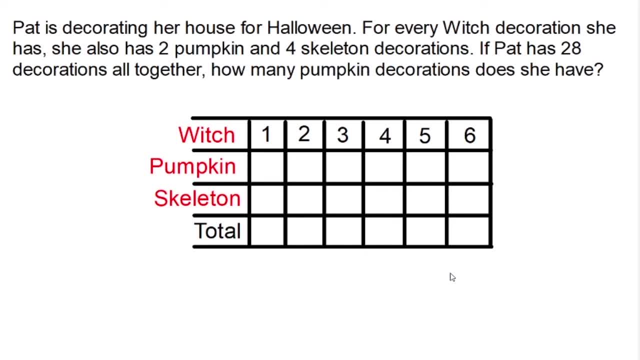 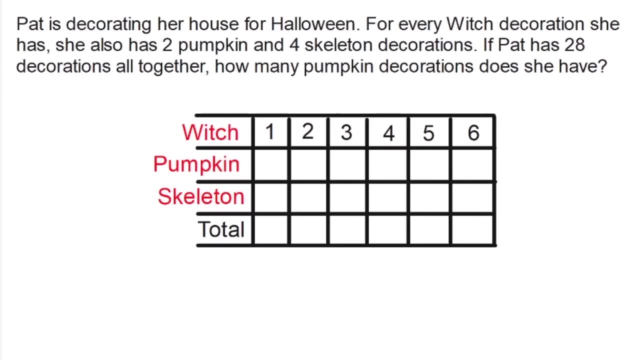 We're going to use this table to solve the problem, So hit pause, Do your best to solve the problem. when you think you got it, Hit play. I'll be here and we'll see how you did. Okay, Welcome back, my friends. 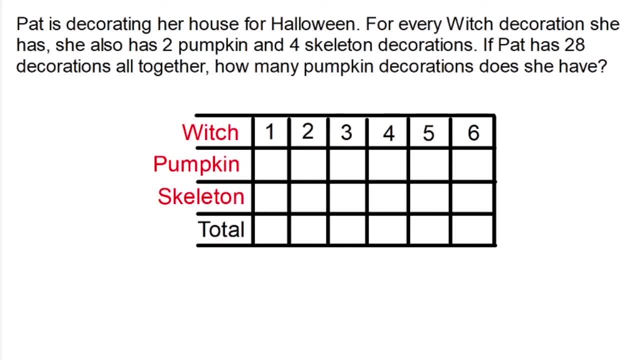 Let's see how you did So. the first thing we need to note is that she has a total of 28 decorations. So when we have a total of 28, we know that we have enough information in our table to solve the problem. But, of course, the first thing we need to do is fill in the table. 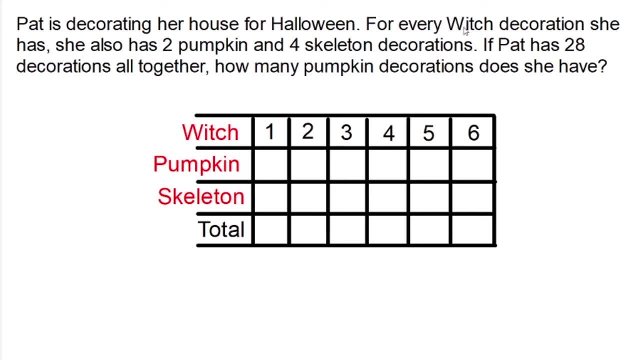 So it says: If she has 41 decorations, that's a witch, She has 2 that are pumpkins and 4 that are skeletons. So with 1 witch decoration that means she has 2 pumpkin decorations and 4 skeleton decorations And in total that makes 7 decorations all together. 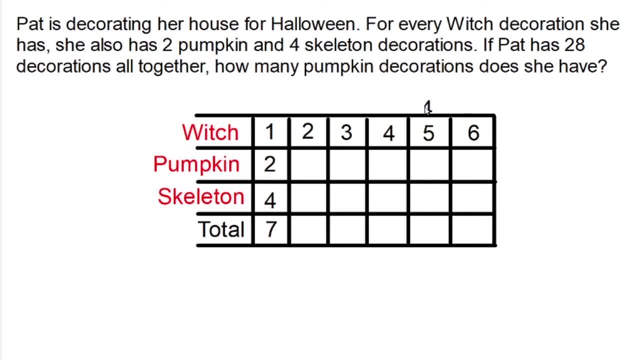 Now, if she had 2 witch decorations, that would mean she would have 4 pumpkin decorations And 8 skeleton decorations, And now she would have a total of 14 decorations all together. Still not enough. We keep going. If she has 3 witch decorations, that means she would have 6 pumpkin decorations and 12. 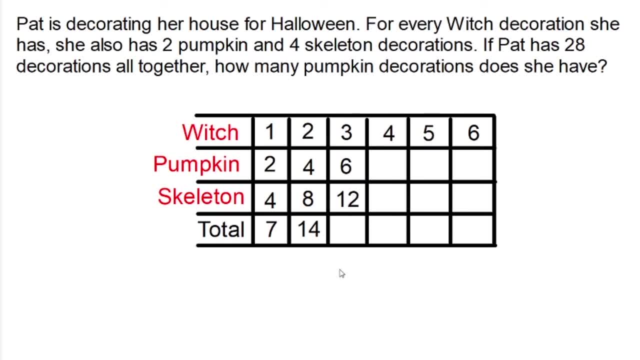 skeleton decorations, And now she would have a total of 20.. So we're going to have a total of 8. And now she would have a total of 21 decorations. Let's keep on going With 4 witch decorations. that means she would have 8 pumpkin decorations and 16 skeletons. 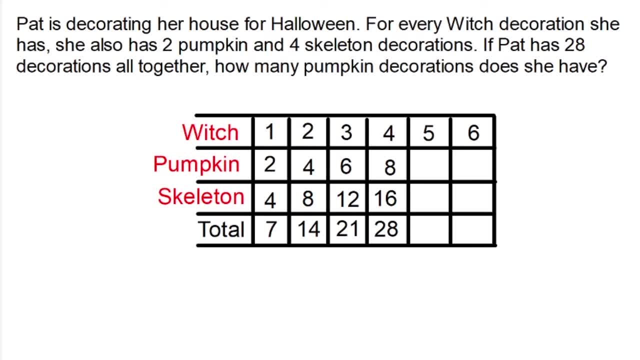 And now she has a total of 28 decorations all together. Well, the problem is saying 28.. We got 28 in our table, So we have enough information to solve the problem. They want to know how many pumpkin decorations does she have? 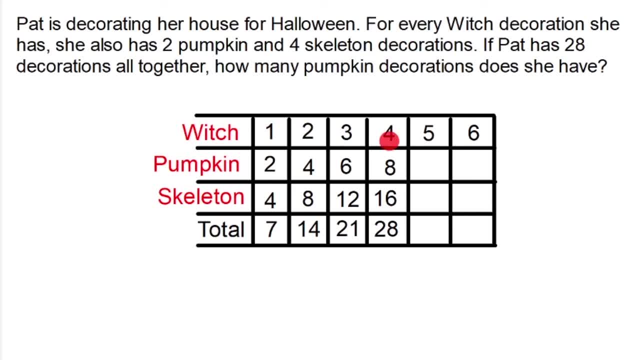 Well, with 4 witch decorations, she has a total of 28 decorations, And of those 28 decorations, 8 of them are pumpkin. So the solution to our problem is: Pat has 8 pumpkin decorations. So how'd you do? Did the table help you solve a problem? 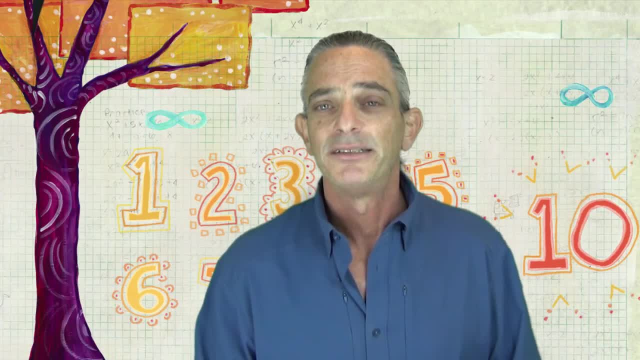 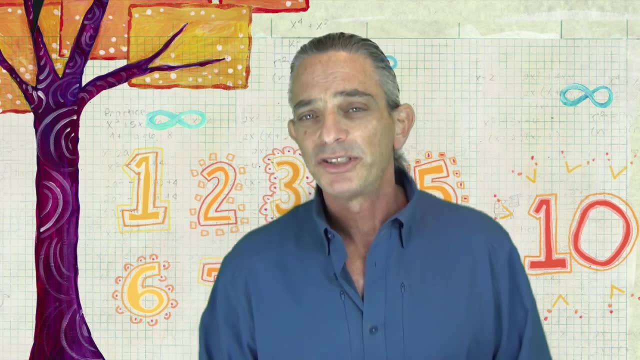 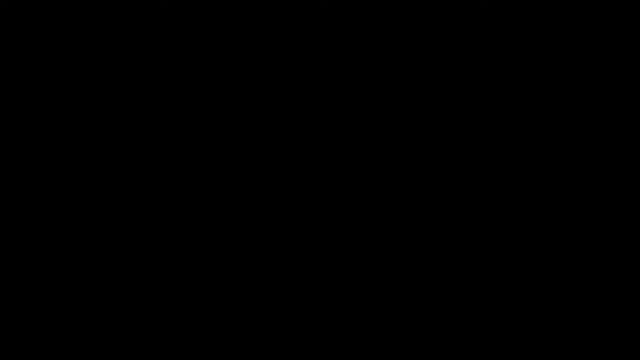 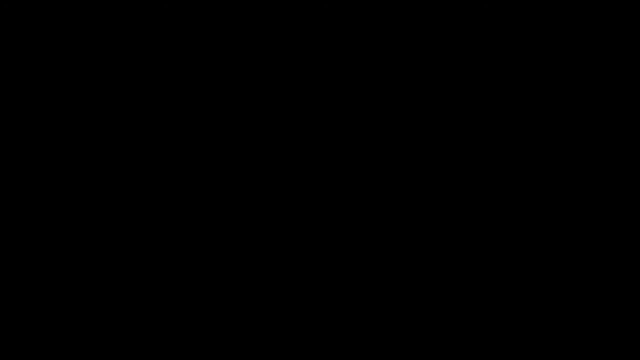 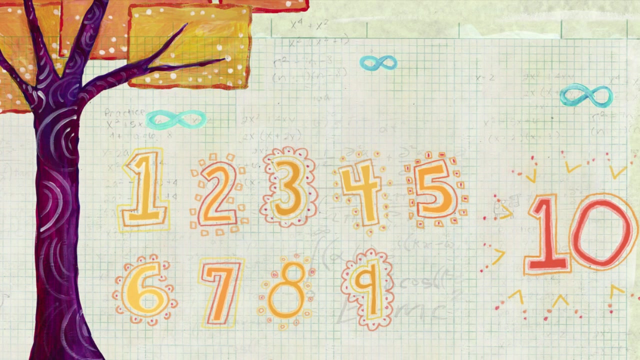